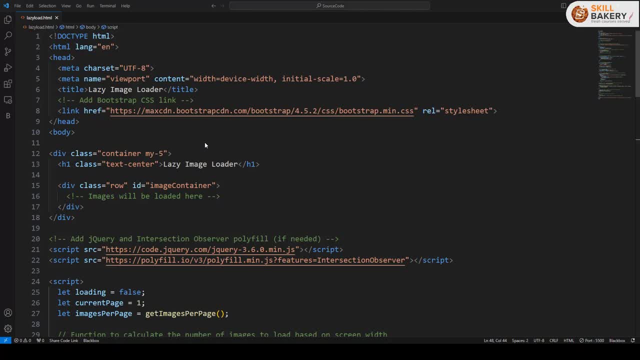 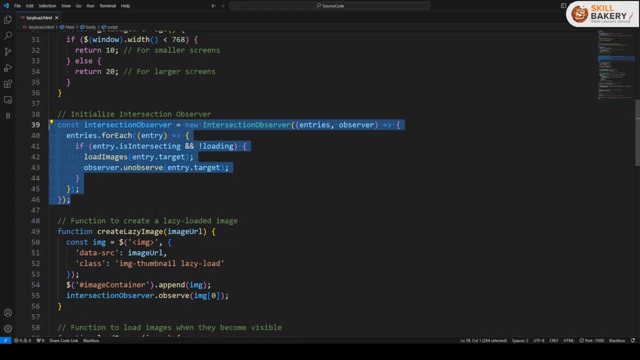 viewport, improving page performance and user experience. Let's start by understanding what the Intersection Observer does. The Intersection Observer is an API that allows us to efficiently track when an element enters or exits the viewport. It is especially useful for implementing lazy loading for images. 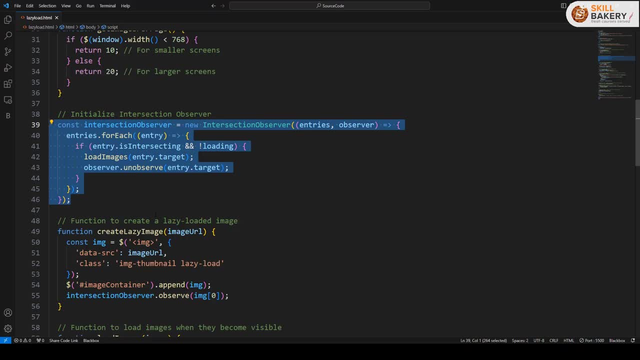 With the Intersection Observer, we can delay the loading of images until they are needed, conserving bandwidth and speeding up page load times. Benefits of Intersection Observer include improved page load performance, better use of network resources and a smoother user experience, especially on pages with many images. now let's dive into how we have implemented the intersection. 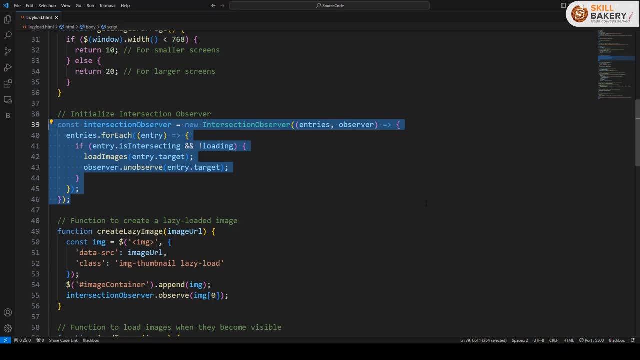 observer. in our code we start by initializing the intersection observer. this is a key part of the lazy loading mechanism. it helps us load images as they become visible on the screen. within the intersection observer we have a callback function. this function is executed when an observed element enters or exits the viewport. so here we have entry dot is intersecting and based on that we 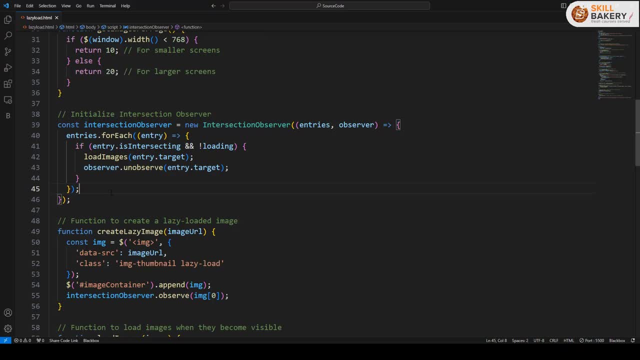 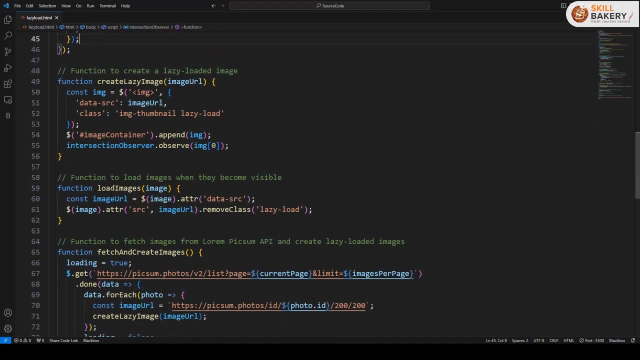 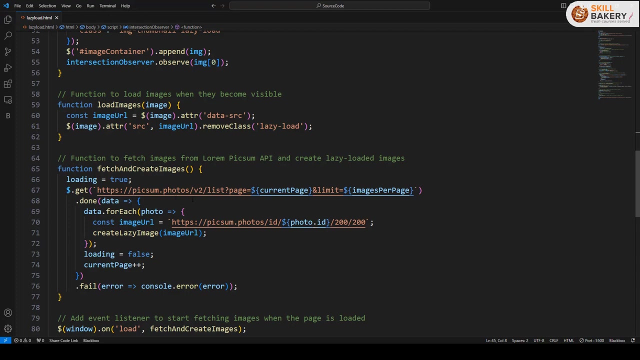 are loading the images. next let's discuss how we fetch and load the images. for that we have a couple of methods, like fetch and create images. that is over here. so here we are making use of pixum photos, api to retrieve random images and it creates lazy loaded image elements. 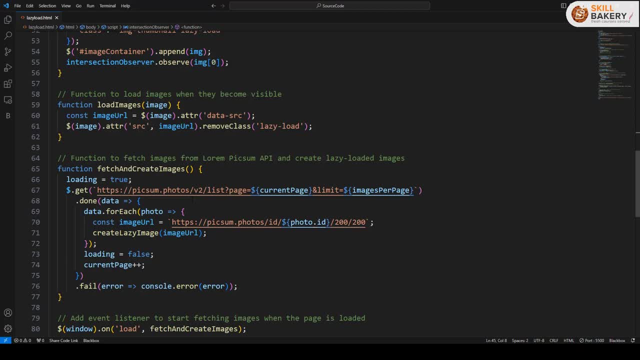 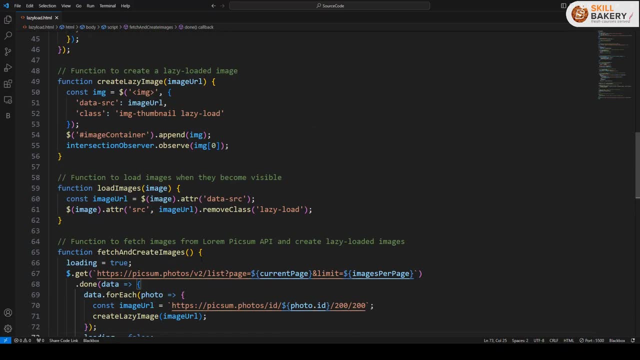 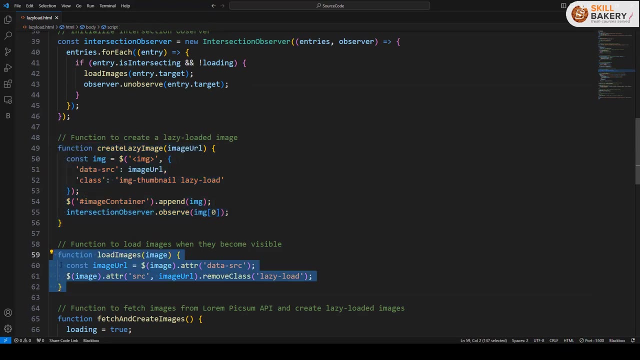 this function is called when the intersecting observer detects that an image is in or near the viewport. then we have this create lazy image and load images function. so here we have the create lazy image and load images function. these two functions are for creating lazy loaded images and loading them when they become visible. this is where the intersection. 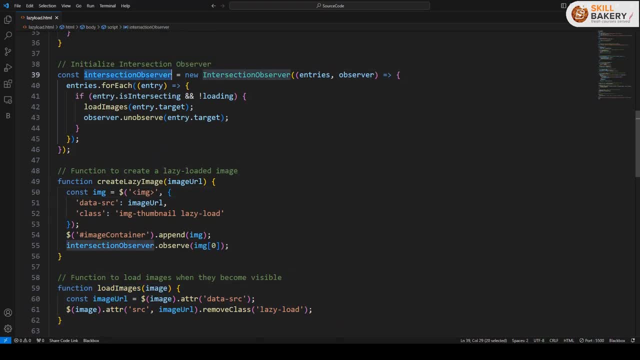 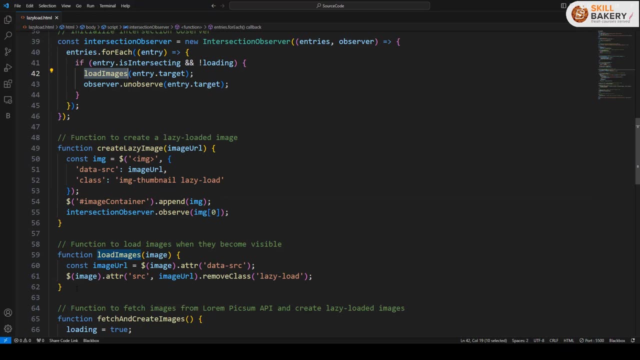 observer is directly involved. so you can see that in our intersection observer we are calling this method load images and that is what we have defined over here. now let's take a look at the event listeners in our code. so we have a window dot to scroll if you scroll down over here, and window dot load. so for